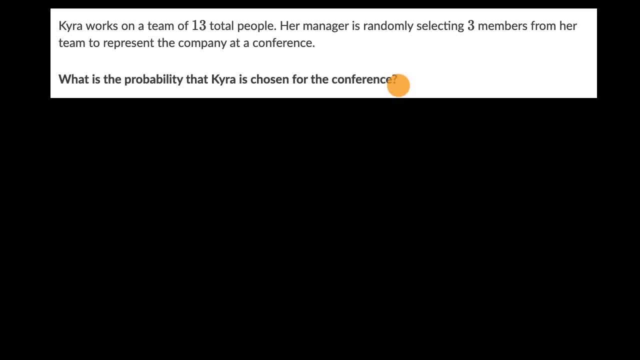 before we work through this together. All right, now let's work through this together. So we wanna figure out this probability, And so one way to think about it is: what are the number of ways that Kyra can be on a team, or the number of possible teams, teams with Kyra? 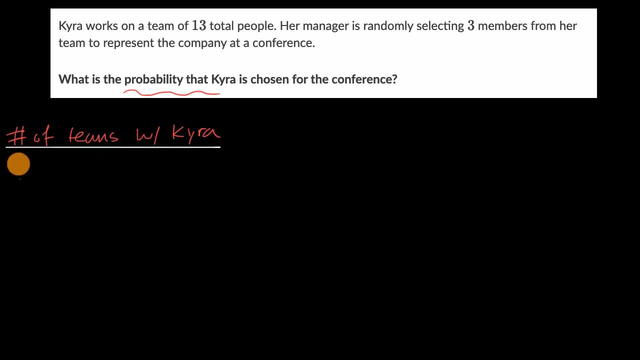 and then over the total number of possible teams. total number of possible teams. And if this little hint gets you even more inspired, if you weren't able to do it the first time, I encourage you to try to pause it again and then work through it. 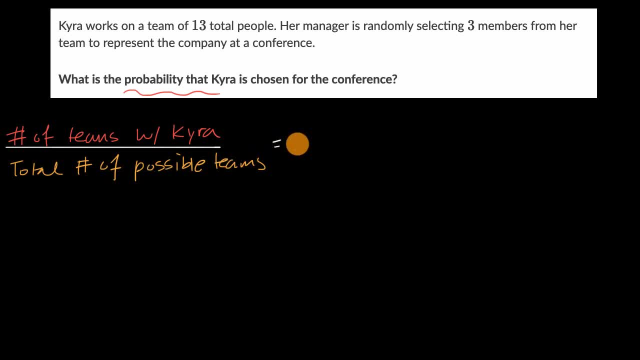 All right, now I will continue. So first let me do the denominator here. What are the total possible number of teams? Some of y'all might've found that a little bit easier to figure out. Well, we know that we're choosing from 13 people. 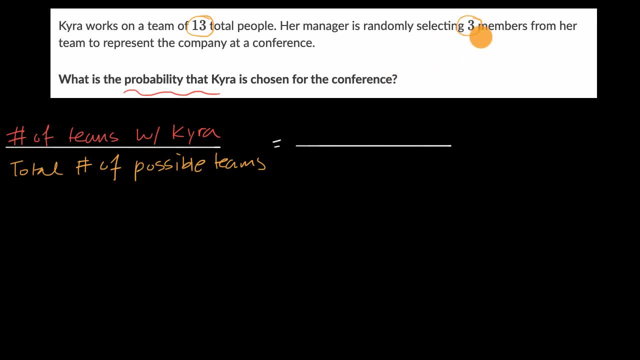 and we're picking three of them and we don't care about order. It's not like we're saying someone's going to be president of the team, someone's going to be vice president and someone's going to be treasurer. We just say there are three people in the team. 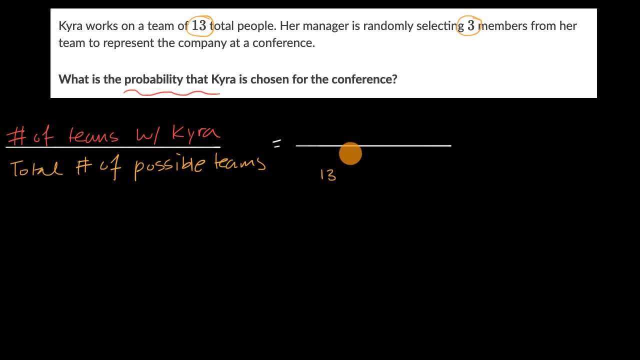 And so this is a situation where, out of 13, we are choosing, we are choosing three people. Now, what are the total number of teams, possible teams that could have Kyra in it? Well, one way to think about it is: 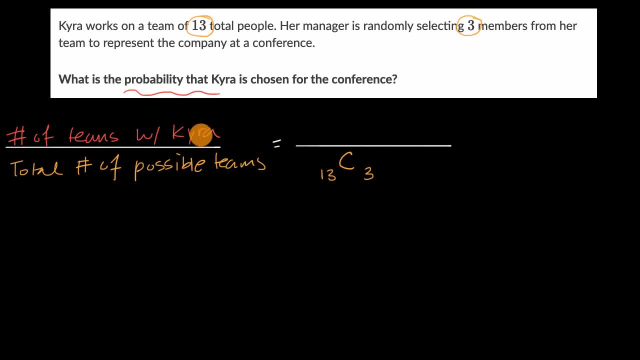 if we know that Kyra's on a team, then the possibilities are: who's going to be the other two people on the team And who are the possible candidates for the other two people? Well, if Kyra's already on the team, 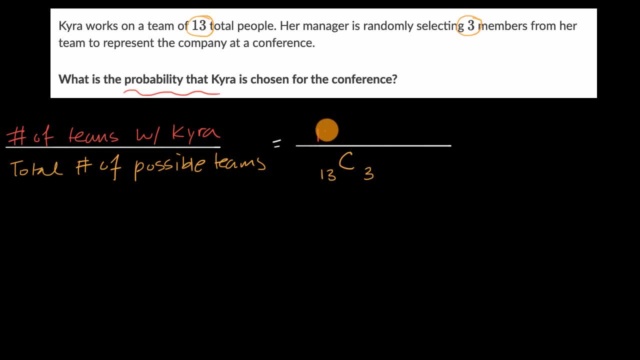 then there's a possible 12 people to pick from. So there's 12 people to choose from for those other two slots, And so we're going to choose two, And once again, we don't care about the order with which we are choosing them. 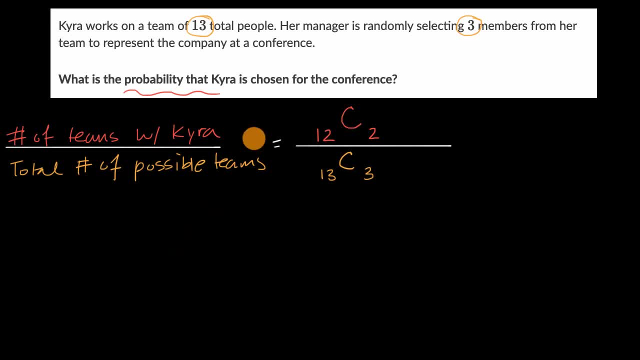 So once again, it is going to be a combination, And then we can just go ahead and calculate each of these combinations here. What is 12? choose two. Well, there's 12 possible people for that first non-Kyra seat. 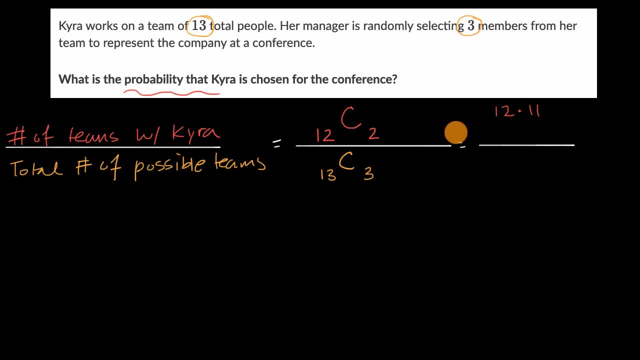 And then there would be 11 people there for that other non-Kyra spot, And of course it's a combination. We don't care what order we picked it in. And so there are two ways to get these two people. We could say two factorial.